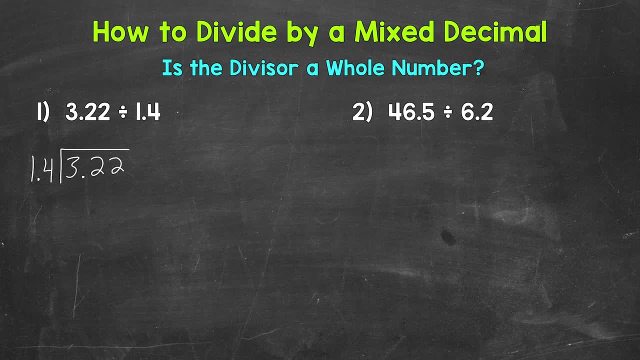 That means we need to make it a whole number. We do this by multiplying the divisor by a power of 10. This will shift the digits to the left and make the divisor whole. Now we can make that very simple and just think of this as moving the decimal to make the divisor whole. 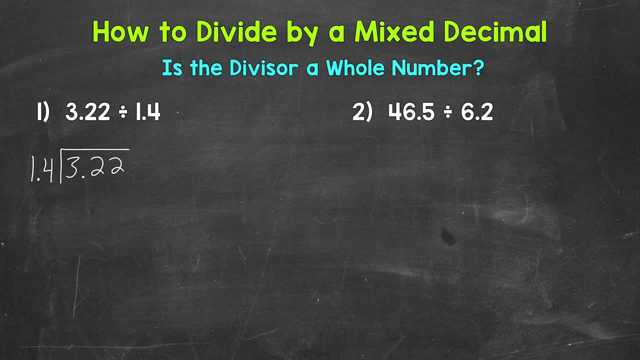 For example, let's move This decimal One place to the right, So it goes after the 4 and we have a whole 14.. Now, whatever we do to the outside the divisor, we must do to the inside the dividend. 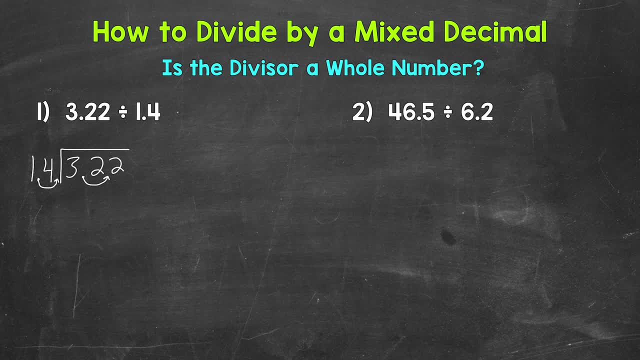 So let's move this decimal once to the right as well. Now again, technically, we multiply the divisor and dividend by a power of 10 to shift the digits to the left and make the divisor whole. For example, we multiplied the divisor by 10 for number one. 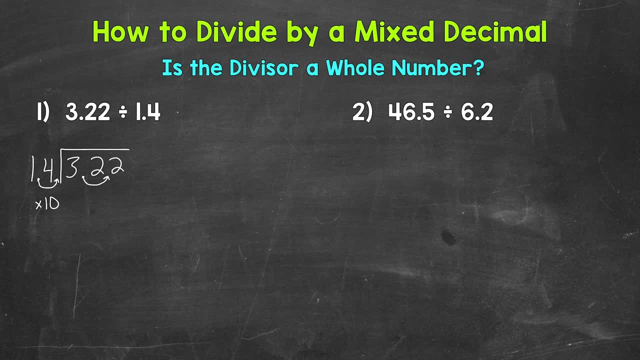 in order to make it whole. That shifted the digits one place to the left and again gave us that whole divisor. We then needed to multiply the dividend by 10 as well. We made this process simpler to think through by just thinking of this as moving the decimal to make the divisor whole. Whatever we 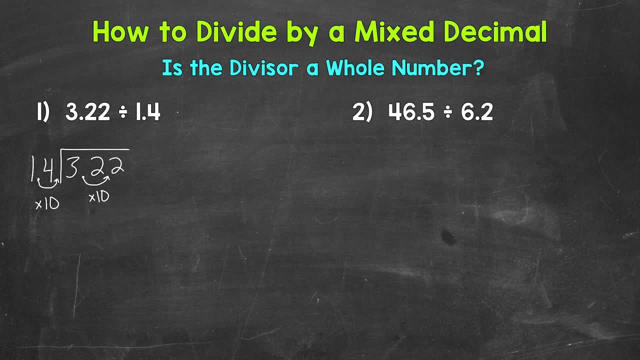 do to the divisor, we must do to the dividend. Making the divisor whole places the decimal for us in our answer and since our divisor is now whole, we can go through our division process, The same process we use with whole numbers. So divide, multiply, subtract, bring down, repeat. 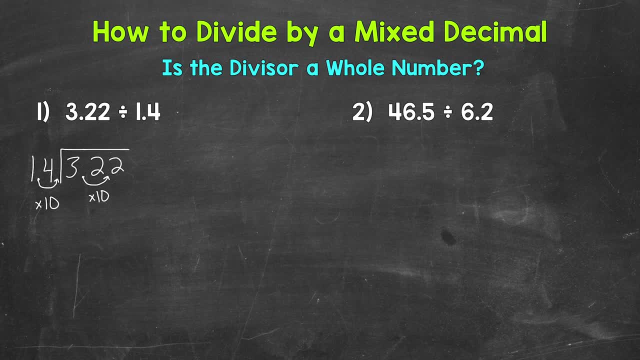 Now we need to rewrite our new equivalent problem with the whole divisor. So our dividend is 32 and 2 tenths divided by 14.. Now, as far as our new equivalent problem, is the divisor a whole number? Yes, so we can bring the decimal straight up into our answer. Now let's go through the division. 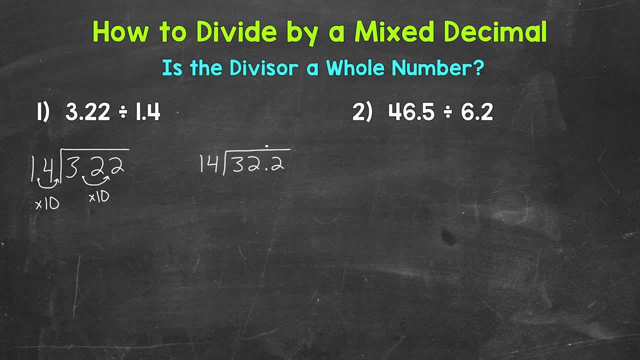 process Starting with divide. So we have 3 divided by 14.. How many whole groups of 14 in 3? Well, we can't do that, So we need to use the 2 and look at 32.. How many whole groups of 14 in 32? Well, 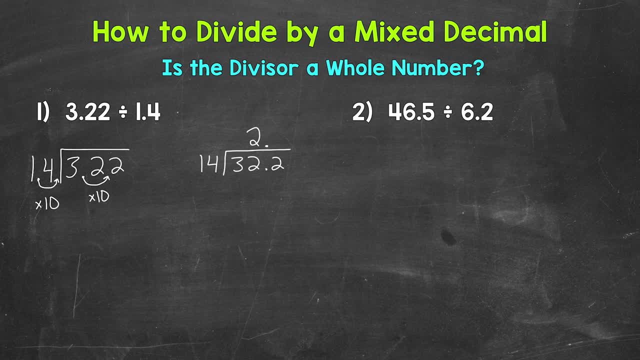 2. That gets us to 28.. So the 2 needs to go above the 2 in 32, not the 3, since we used both the 3 and the 2.. Now multiply 2 times 14. 28. Subtract 2 minus 8.. Well, we need to borrow. So we have 12 minus 8, which is 4.. 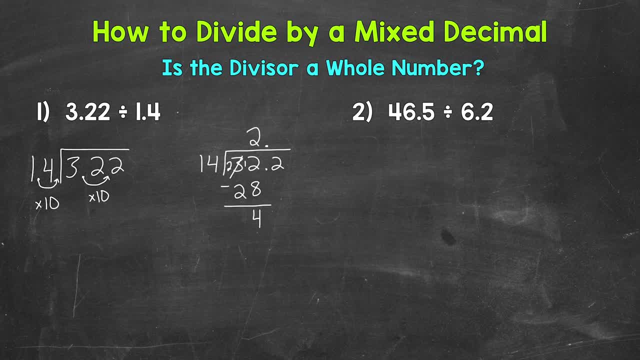 And then 2 minus 2 is 0. So 32 minus 28 equals 4.. Then we bring down, That gives us 42. And we repeat, So we go back to divide. We have 42 divided by 14.. How many whole groups of 14 in. 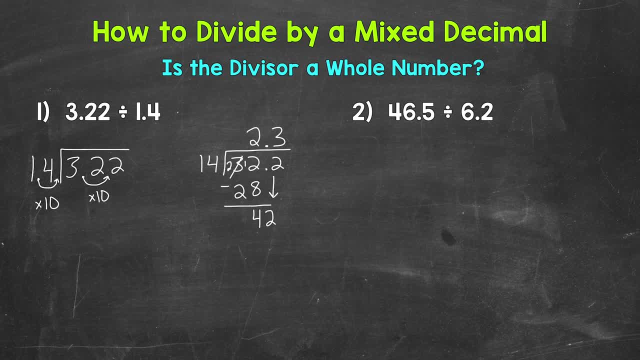 42?? Well, 3.. That hits 42 exactly. Multiply 3 times 14.. 42. Subtract 42 minus 42 is 0.. We went all the way over to the right within our dividend as far as bringing digits down. 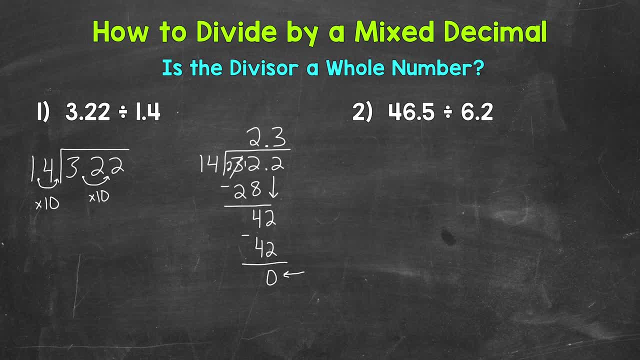 And we have a clean cut, 0 at the end. So we are done. Our final answer: 2 and 3 tenths. Let's move on to number 2, where we have 46 and 5 tenths divided by 6 and 2 tenths. Let's set this: 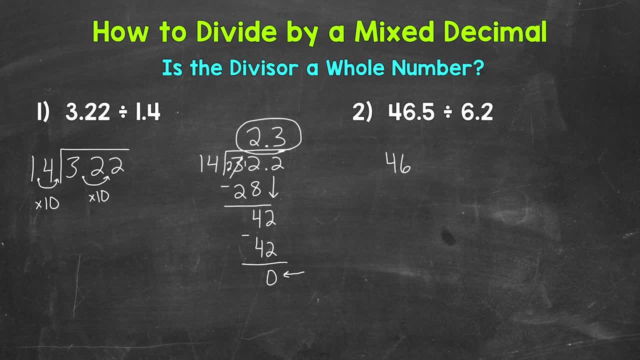 problem up: 46 and 5 tenths is the dividend. the number we are dividing 6 and 2 tenths is the divisor, the number we are dividing. by Now that we are set up we need to check: Is the divisor a. 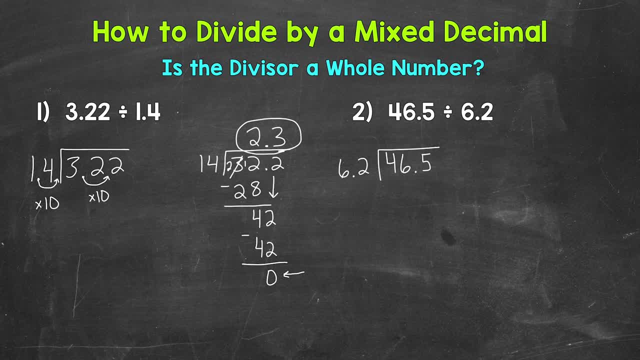 whole number. We need to check: Is the divisor a whole number? We need to check: Is the divisor a whole number? 6 and 2 tenths is not a whole number, So let's make it a whole number. Let's. 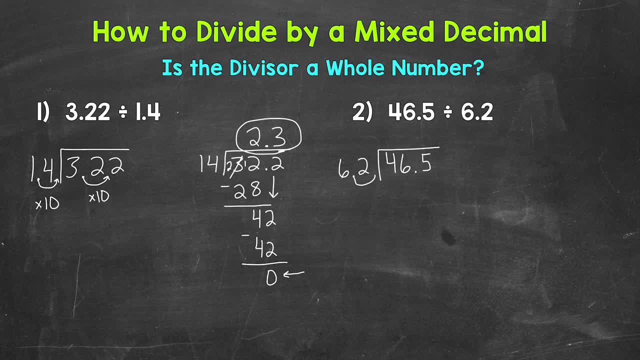 move the decimal once to the right, So now we have a whole 62. Technically, we multiplied our divisor by 10.. That was the power of 10. we multiplied the divisor by Now. whatever we do to the outside the divisor, we must do to the inside the dividend. So let's move this decimal. 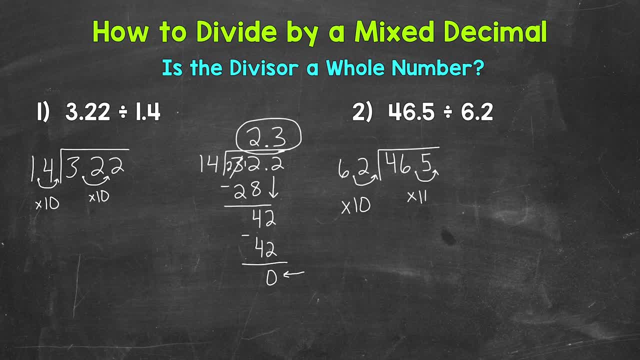 once to the right as well, And again, technically, we are multiplying our divisor and dividend by 10. Now we have a whole divisor, so we can rewrite our equivalent problem. We have 465 divided by 62. Now that we have our rewritten equivalent problem with a whole divisor. 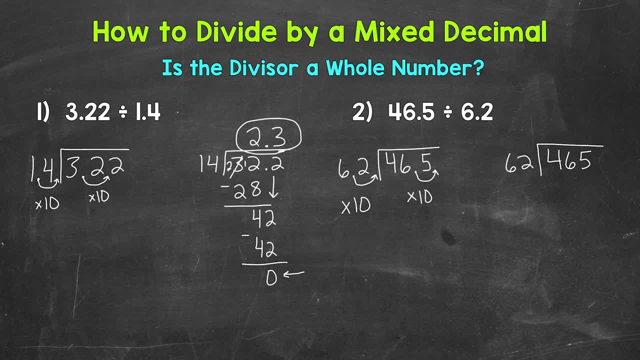 we can go through the division process. So we have 4 divided by 62.. How many whole groups of 62 in 4?? Well, we can't do that, So we need to use the 6 and take a look at 46.. How many whole groups of 62 in 46?? Well, we can't do that either. 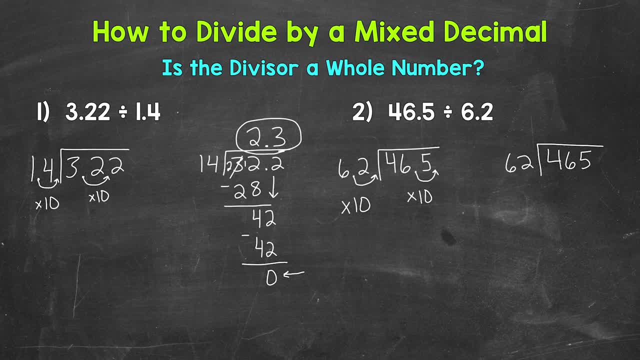 So we need to use the 5 and take a look at 465.. How many whole groups of 62 in 465? We're going to need to estimate and check in order to figure out how many whole groups of 62 in 465.. So let's. 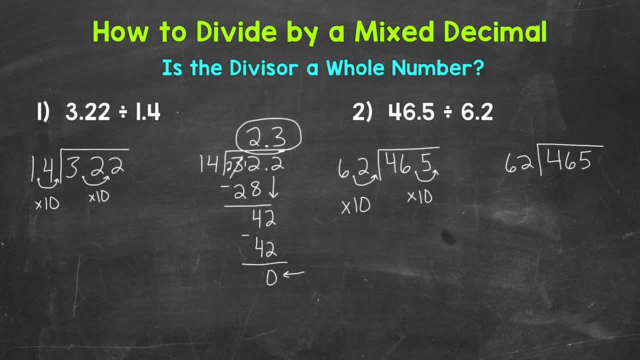 figure this out, because I don't know how many whole groups of 62 are in 465.. So let's come to the side and again estimate and check. I'll use 62 times 10 as a reference, a starting point. We. 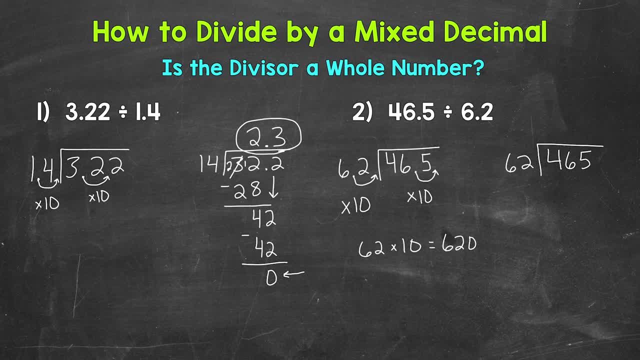 know, 62 times 10 is 620.. That gives us something to go off of. We can base our first estimate off of 620 and go home. So let's go ahead and do that. So let's go ahead and do that. So let's go ahead. 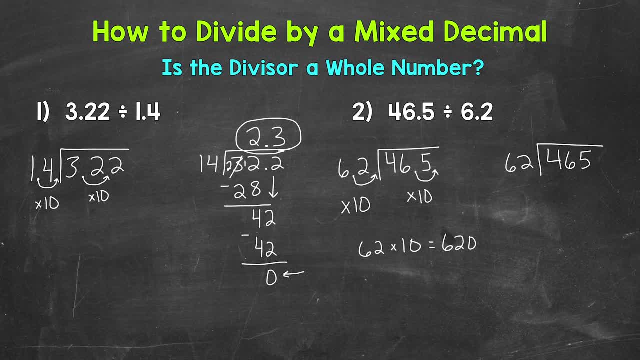 from there. 465 is less than 620, but it's kind of close. So let's back up from 10 and try 62 times 8 and see how close we get. So let's multiply 62 times 8 and again see how close we get We are. 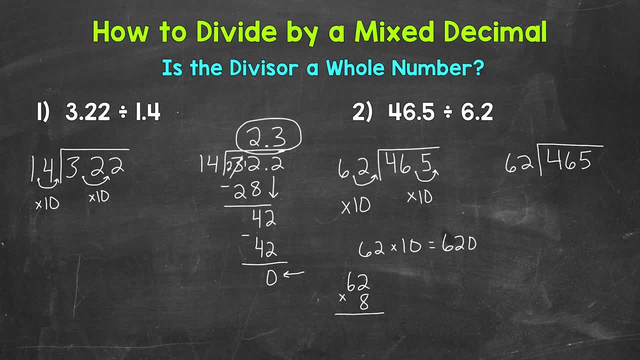 estimating and checking: 8 times 2,, 16.. 8 times 6,, 48 plus 1. 49.. So we get 496, which is too much, So we need to back it up. Let's try 7.. 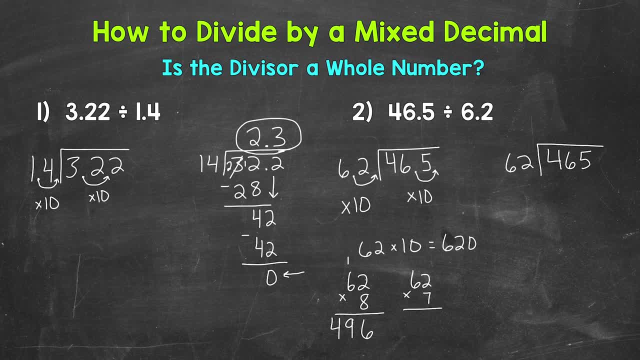 62 times 7.. 7 times 2, 14.. 7 times 6, 42 plus 1, 43. So 434.. It's going to be 7 whole groups of 62. So put the 7 above the 5, since we used 465.. Now multiply 7 times 62,. 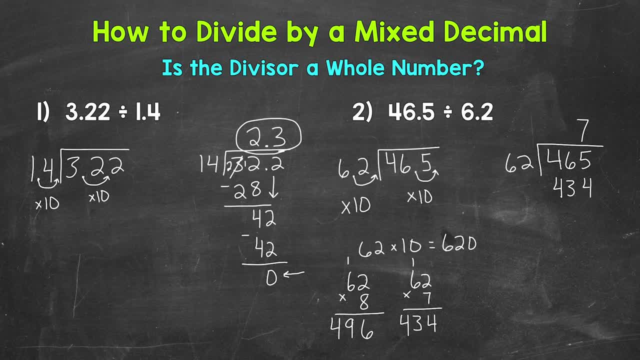 434.. Subtract: 5 minus 4 is 1.. 6 minus 3 is 3.. 4 minus 4 is 0.. So we get 31.. So 465 minus 434 equals 31. 31.. Now we are at the bring down step, but there's nothing else to bring down And we don't. 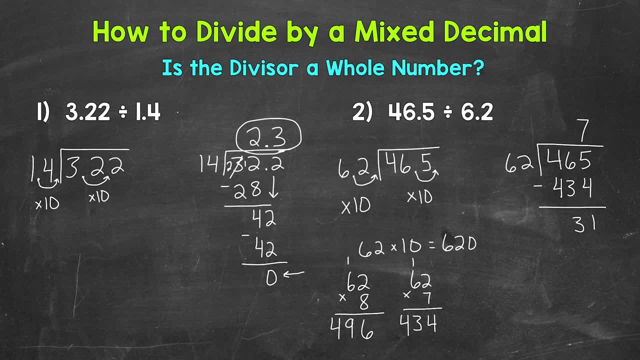 want to write 7, remainder 31.. We are working with decimals So we want to keep everything in decimal form, even the answer. So we need to continue this problem. So what we can do, we can place the decimal in our dividend. A decimal comes after a whole number, So after 465.. 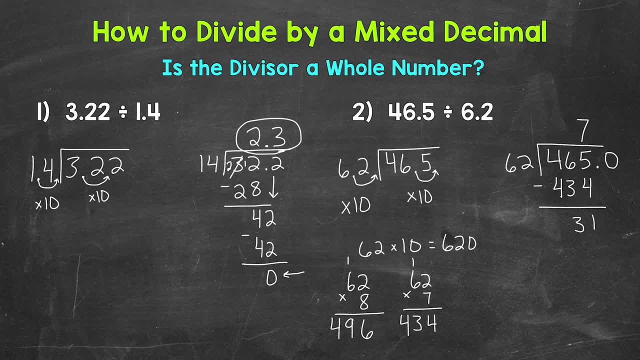 Then we can Write a 0 in the tenths place. Now we're able to bring that 0 down and continue the problem. That 0 to the right of a decimal does not change the value of the problem. We still have 465.. 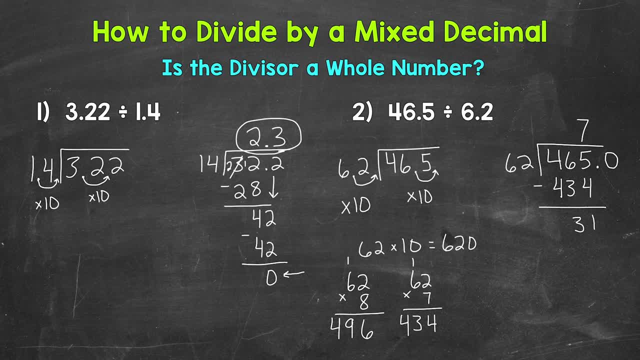 So we are able to do this. Once we place the decimal and write the 0, we can bring the decimal straight up into the answer and bring the 0 down. We have 310 and we repeat, So we go back to divide 310 divided by 62. How many whole groups of 62 in 310?? 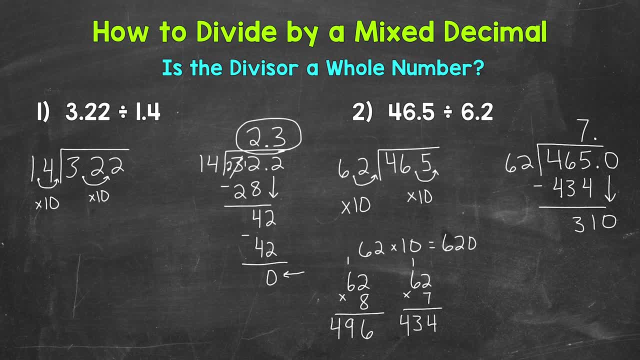 Well, 310 is exactly half of 620.. So it's going to be 5.. But let's come to the bottom and make sure Let's do 62 times 5.. 5 times 2 is 10.. 5 times 6 is 30.. Plus 1 is 31.. 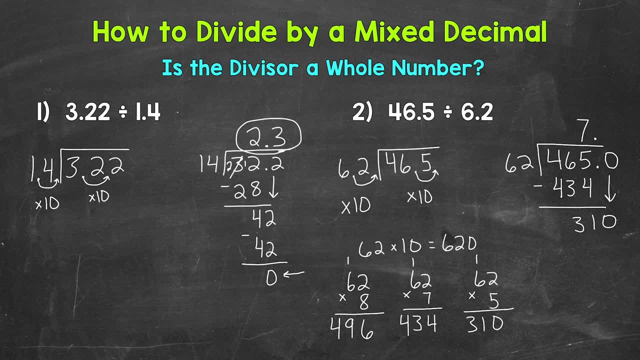 so five whole groups of 62 hits 310 exactly. so let's put our five up here and we can extend this division bar. multiply five times 62, 310, subtract, we get that clean cut zero. we went all the way over within our dividend and we have a clean cut zero at the end. so we are done seven.